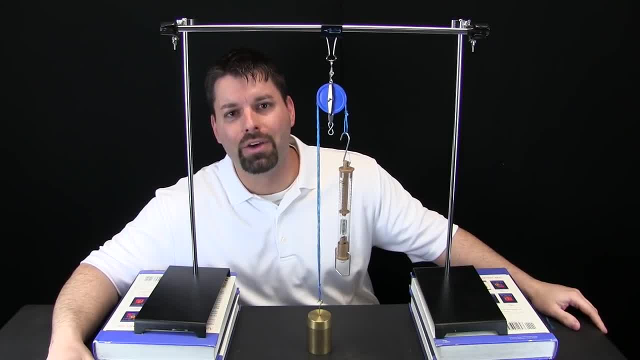 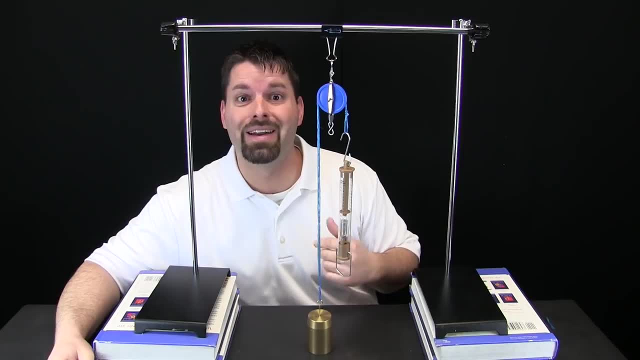 Hi, I am Jared. Welcome to Fun Science Demos. In other videos we talked about simple machines and how simple machines make our work easier. Today we are going to talk about another simple machine called the pulley. And that is a pulley right there. So let us take a. 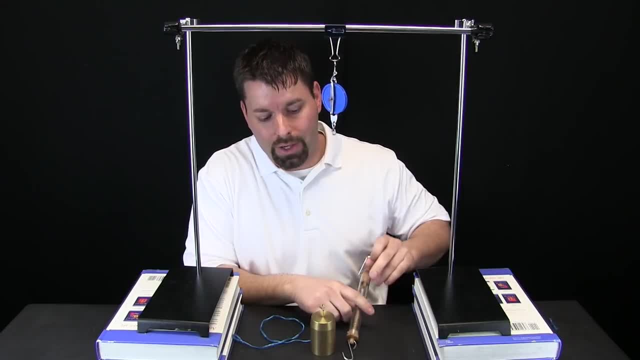 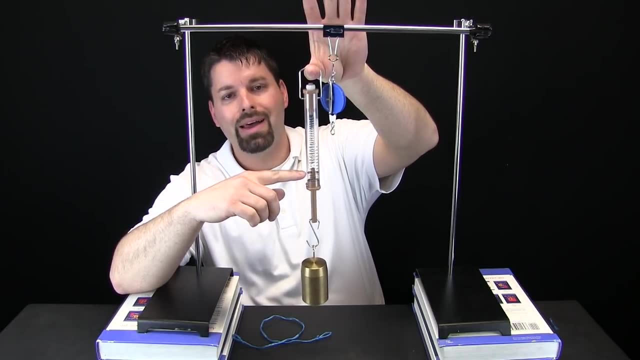 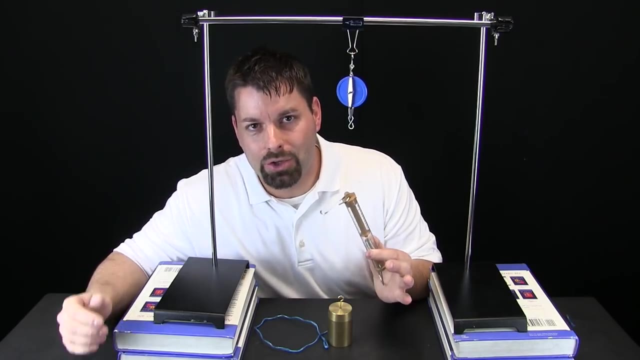 look at our setup. I have a 1000 gram weight and I have a spring scale. If I attach my spring scale to my weight and lift it straight up, it is going to weigh 1000 grams. We can zoom in and take a closer look to see that it weighs 1000 grams. So our spring scale. 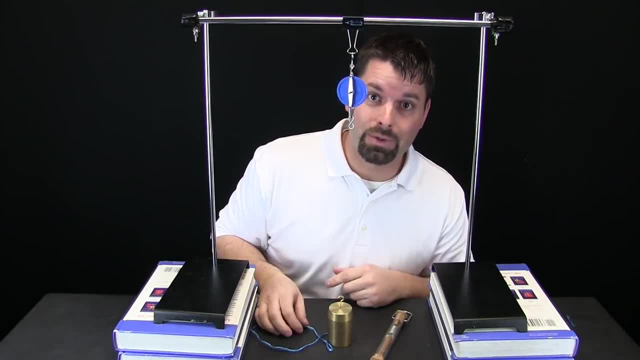 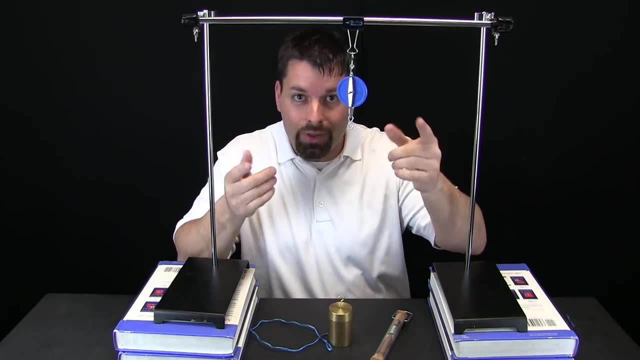 showed us that this 1000 gram weight is really 1000 grams. But we said that simple machines make our work easier. We also said that this pulley is a simple machine. So how do we show you that this pulley makes our work easier? Well, we are going to thread this rope through. 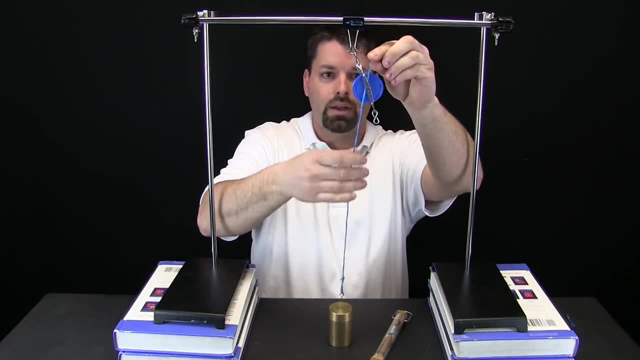 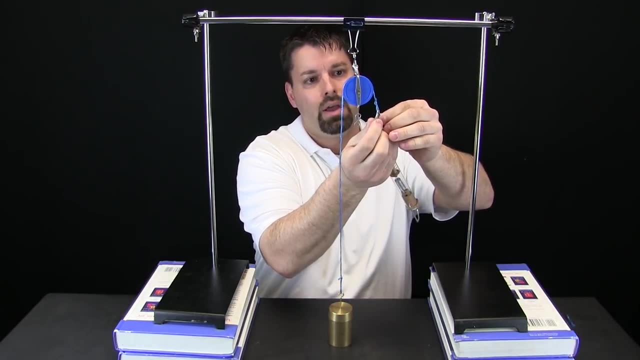 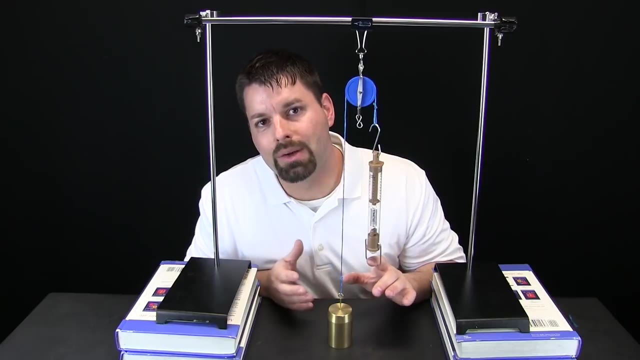 our pulley, attach it to our weight and attach the other end to our spring scale And then pull down the pulley and then pull the weight into our weight, And now we can see if our simple machine, our pulley, really does make work easier. So now it is time to see our 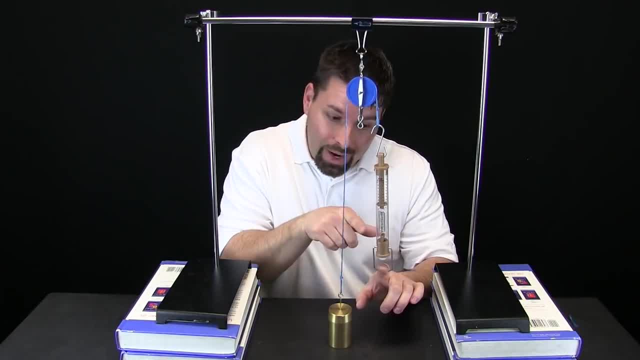 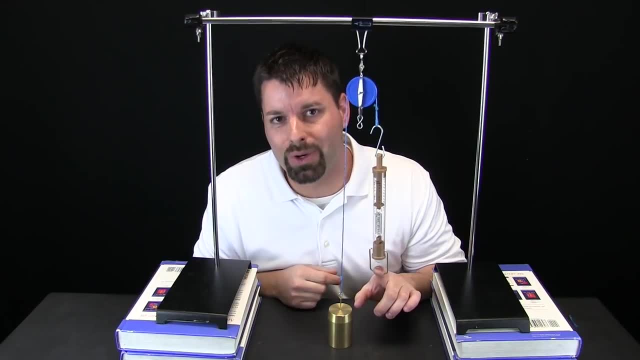 pulley in action. I am going to pull down on the spring scale. When I pull down, the weight should go up, And we are going to see if this pulley has made our work easier by taking a closer look at our spring scale. Here we go: I pull down, the weight goes up. 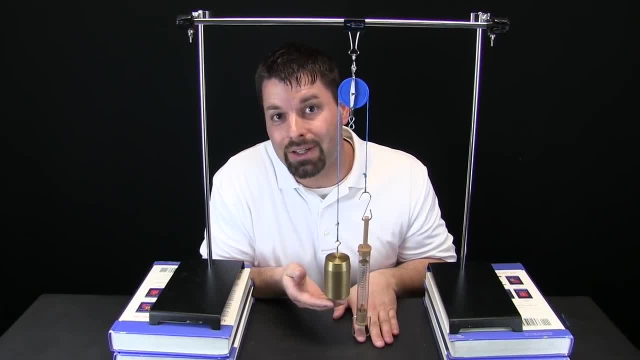 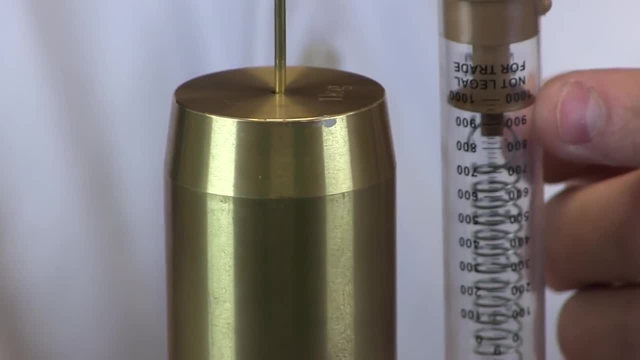 and now we are going to zoom in and take a closer look at our spring scale to see if is making our work easier. So our weight is off the ground and when we look at our spring scale it is just at about 1,000 grams. But wait a second, that really has not made our work that. 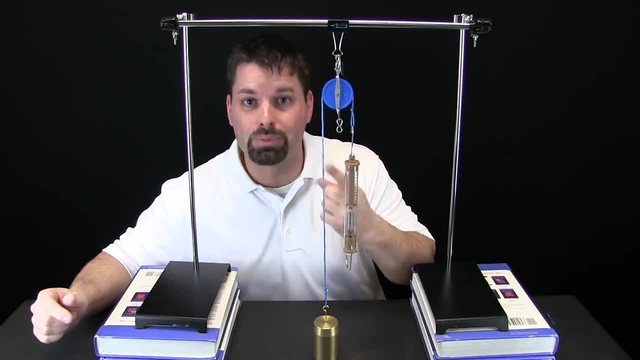 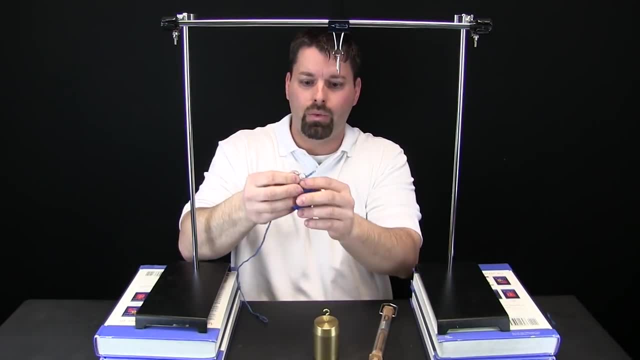 much easier. So let us change this setup and use this pulley differently to see how it works. To do that, I am going to take the pulley off, the scale off and the weight off And I am going to attach the pulley to my weight. 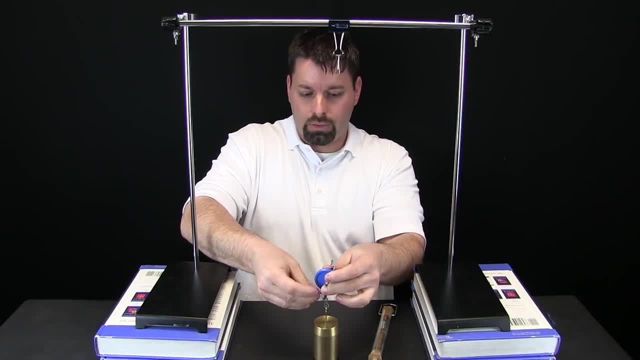 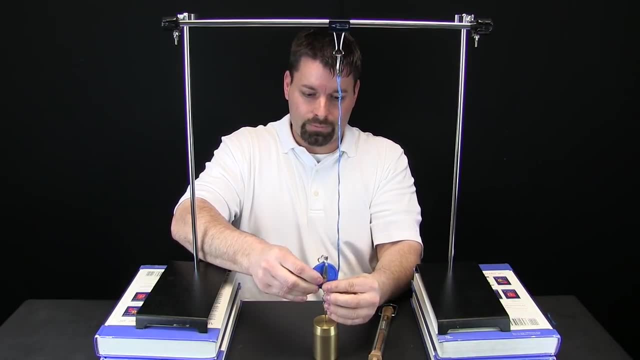 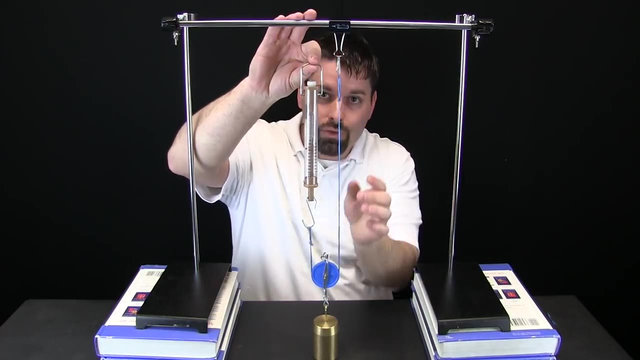 Now I am going to run my rope or my string through and attach my rope to a fixed point above the weight and then attach my spring scale. It kind of looks like I reversed the whole thing around: Instead of the pulley being up top, the pulley is now at the bottom And we are going to 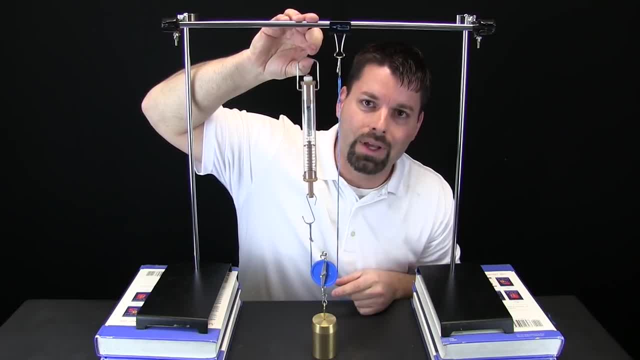 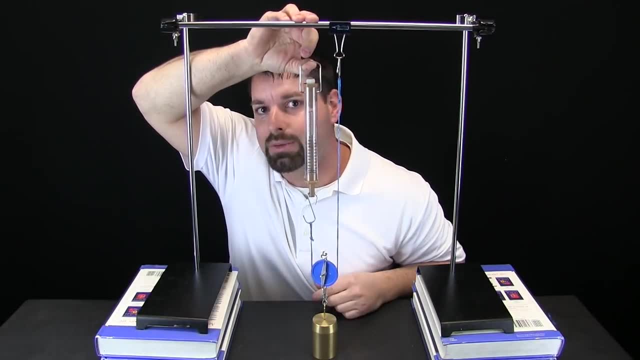 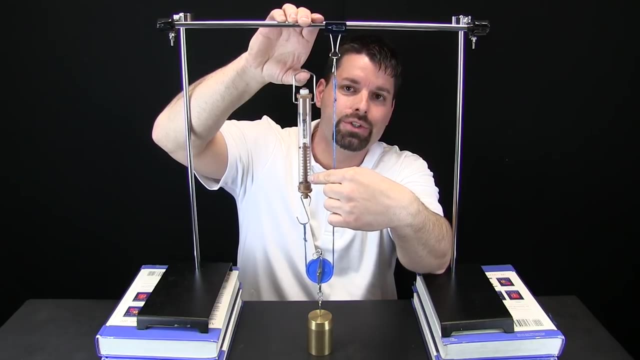 try and lift this weight with the pulley at the bottom and see what happens on our spring scale. We are going to zoom in and take a closer look so you can see if our work really is made easier by using our pulley differently. Right now our spring scale is reading 0 grams. Down here is 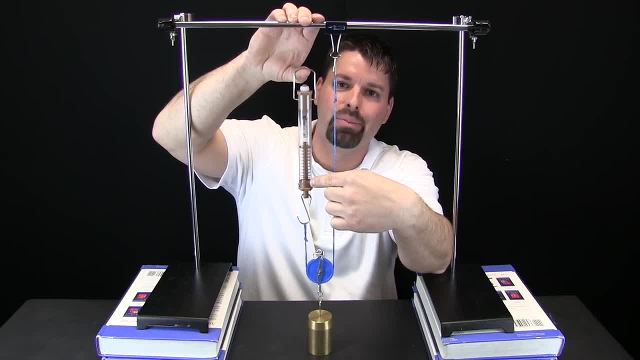 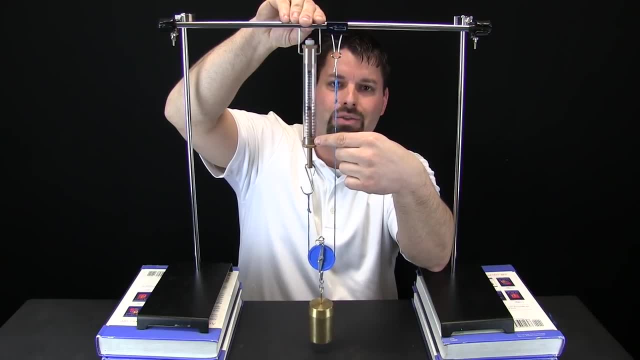 1,000.. Watch what happens carefully to our spring scale when I pull up. I pull up, the weight is off the table, but my spring scale did not go down to 1,000.. We are going to zoom in and take. 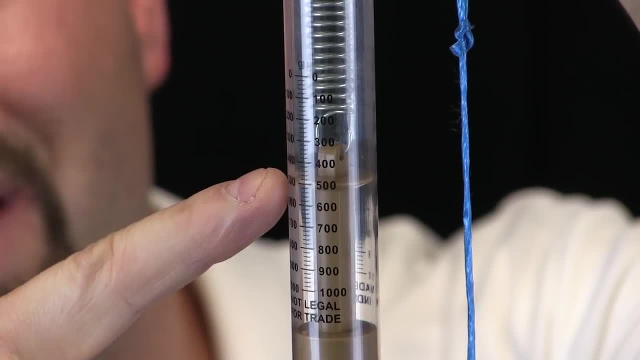 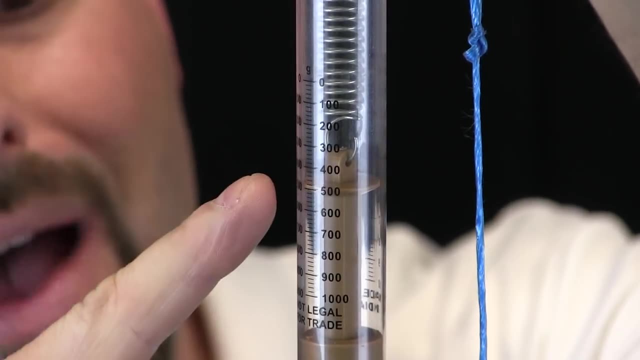 a closer look. So we have zoomed in and we can see that our spring scale is right at 500 grams. I would say this pulley has made our work easier. In our last setup it took about 1,000 grams, but with this setup because we used our pulley. 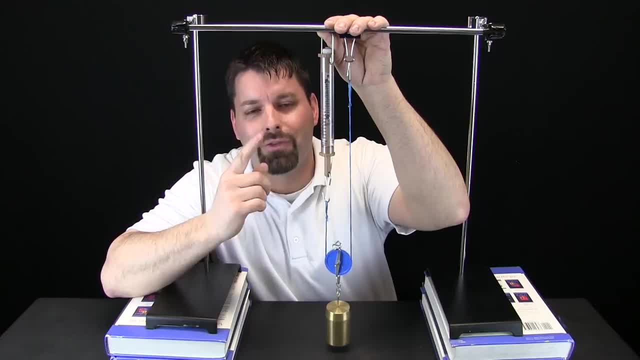 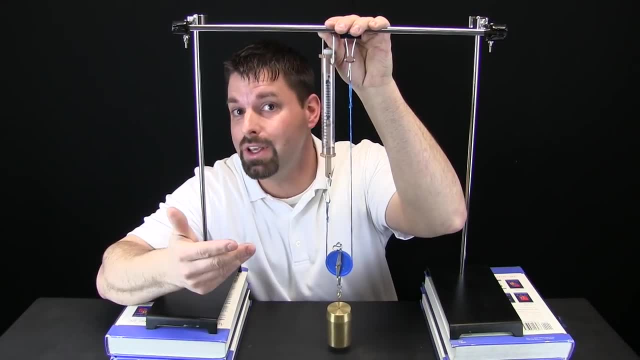 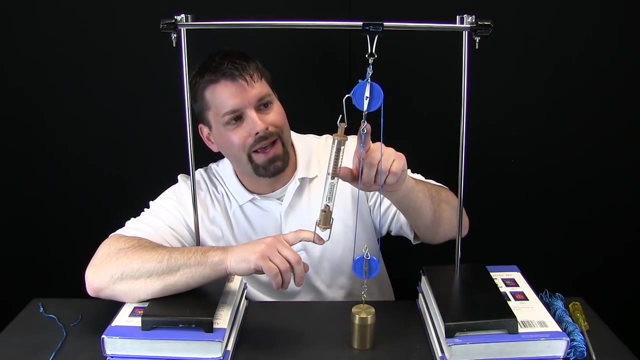 differently. we are at 500 grams. If one pulley can make our work easier, it kind of gets me thinking. I wonder if two pulleys can make our work even easier, What do you think will happen? So now we have two pulleys set up and working together, I have a string attached to my top. 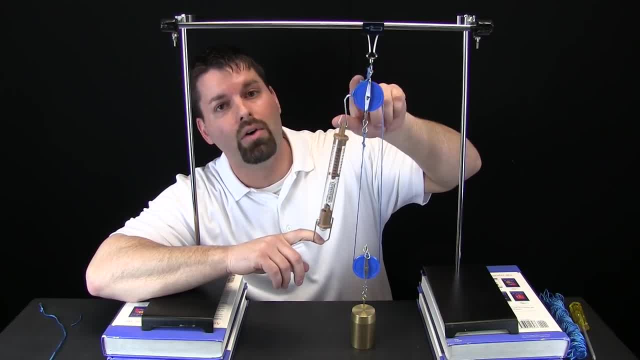 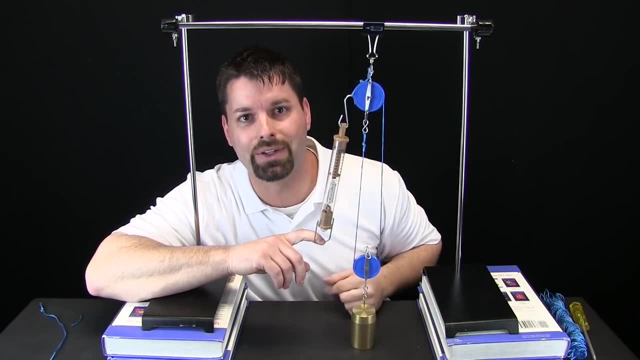 pulley. It comes down around my bottom pulley, up over the top of this pulley, and now I have my spring scale attached And now I can pull down and see if this really does make our work easier. Remember when I had one pulley at the bottom, it was 500 grams. What do you think? 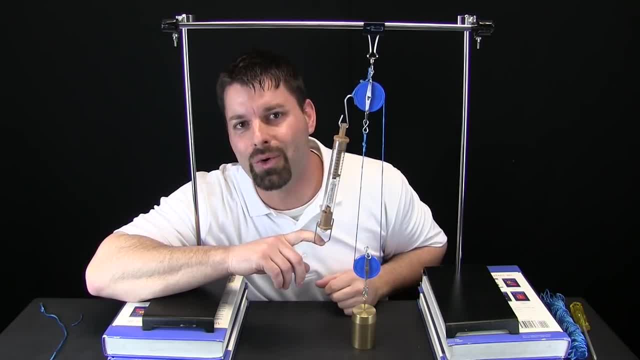 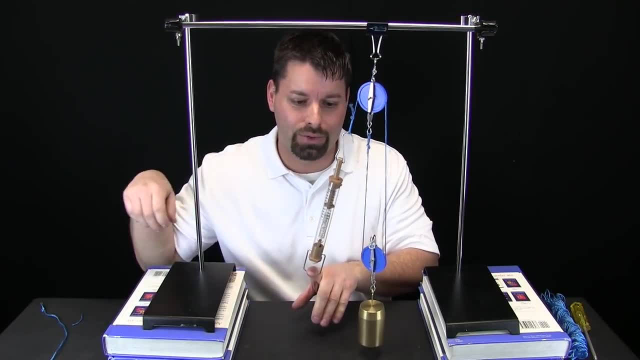 will happen when I pull down? How much do you think our spring scale will read? We are going to pull down on our spring scale and zoom in and take a closer look so you can see what happens. I pulled down, my weight is off the ground and now we are going to zoom in to our spring scale. 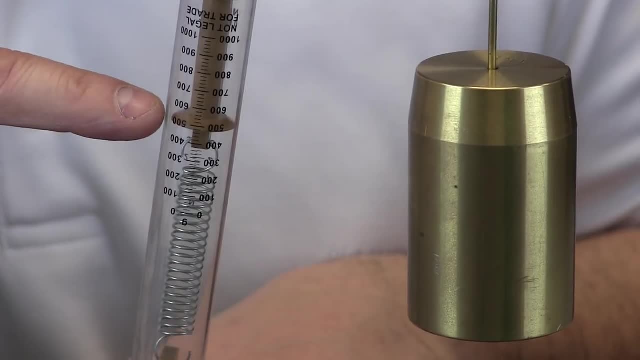 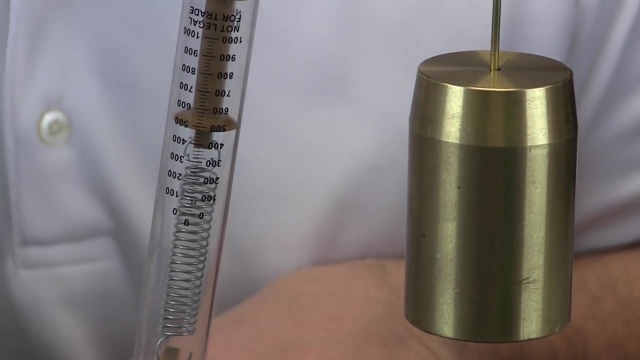 Now that I have this machine right under my front, pulley is right on 500 grams. so did adding a pulley really make that much of a difference? It did not, but remember, adding one didn not make much of a difference, but we used that pulley differently. So I wonder, if we add, 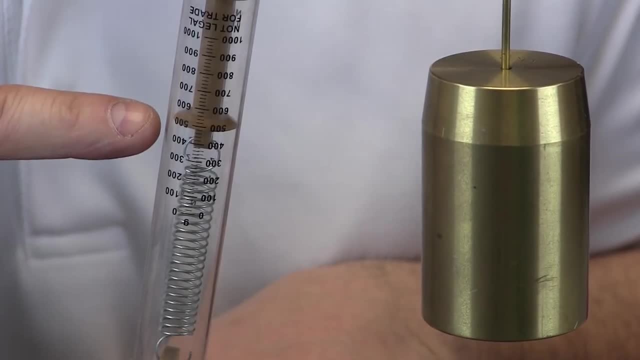 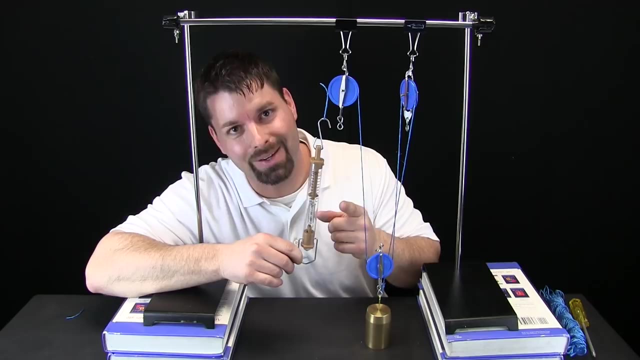 a third pulley, but use it a little differently to see if that will make our work easier. So let us try that. Now we have one, two, three pulleys working together. Try and follow this, because I am going to show you how we set this up. So I have a string. 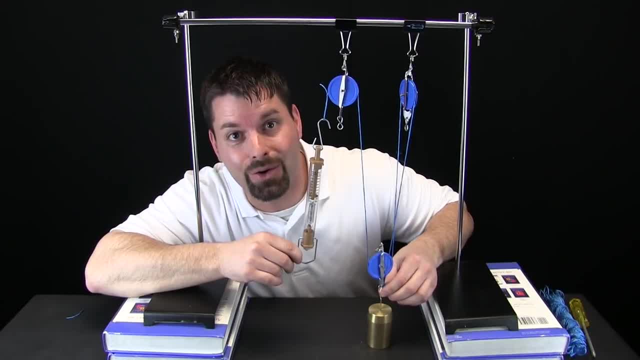 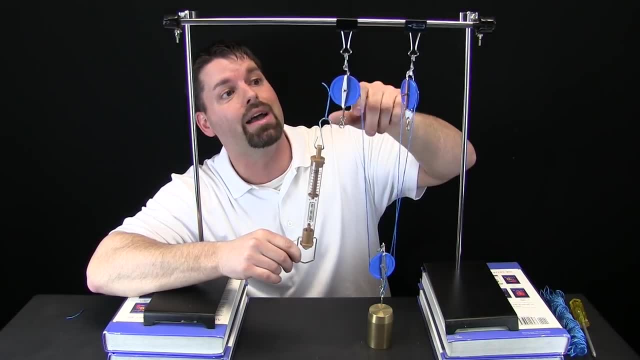 that is attached to my thousand gram weight. Remember it is 1000 grams. The string comes up over top of the first pulley, down around the bottom of the second pulley, back up over top of this third pulley and now. 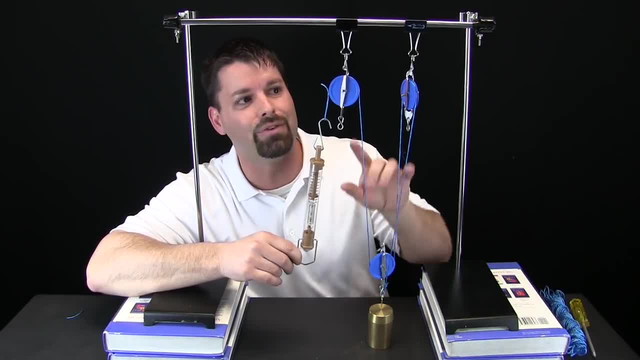 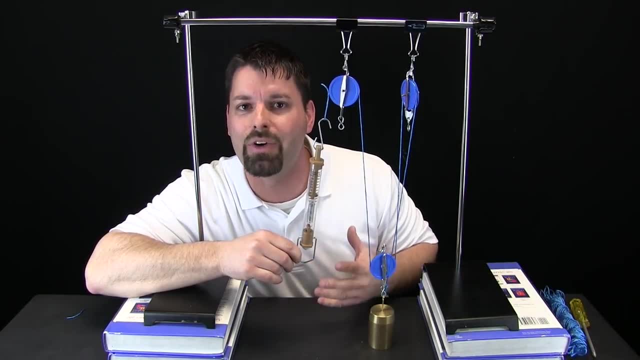 I have my spring scale so we can make sure to check to see if all of these pulleys working together really does make our work easier. Remember when we had two pulleys working together it was about 500 grams. It made our work easier. What is it going to be when we 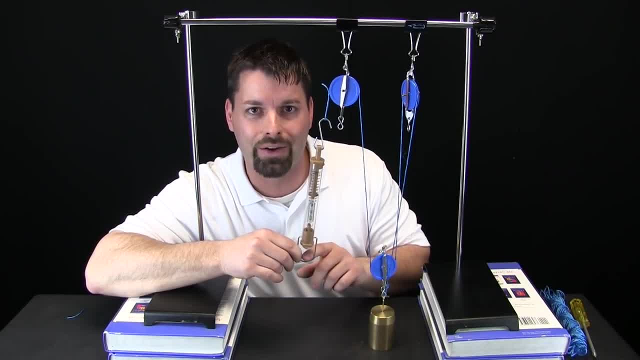 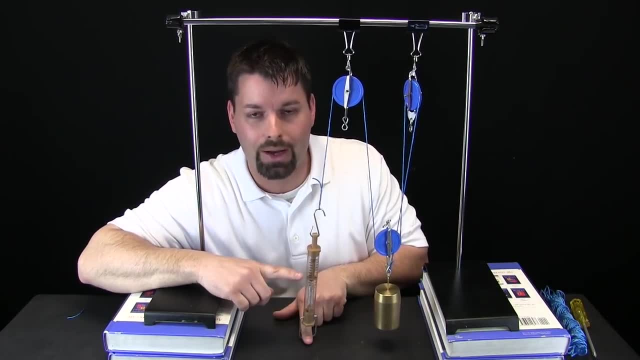 have three pulleys working together. We are going to pull down and see if our spring scale is working and then zoom in and take a closer look. I pull down on the spring scale, my weight comes up and now let us zoom in to see what our spring scale says. Take a look. 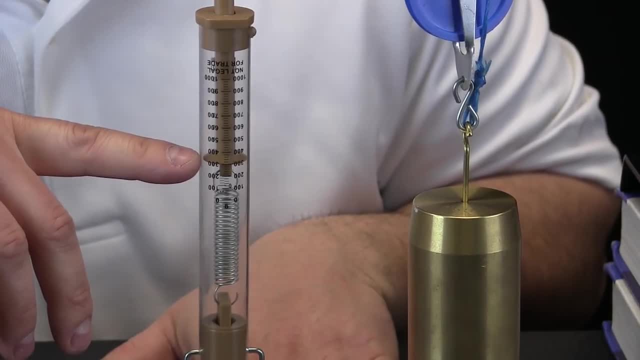 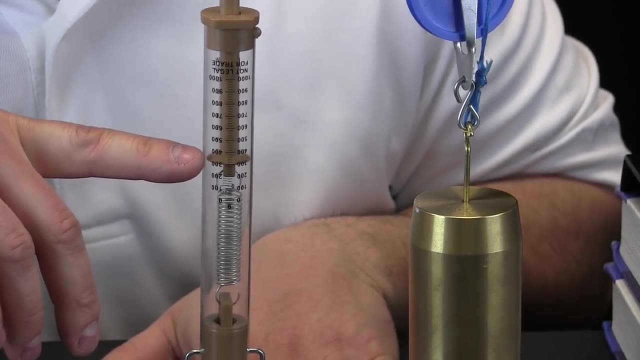 at this: Our spring scale is showing 300 grams. Three pulleys working together that took a 1000 gram weight and now I am only pulling 300 grams. I would say our work is really easier. I wonder what would happen if we put four. 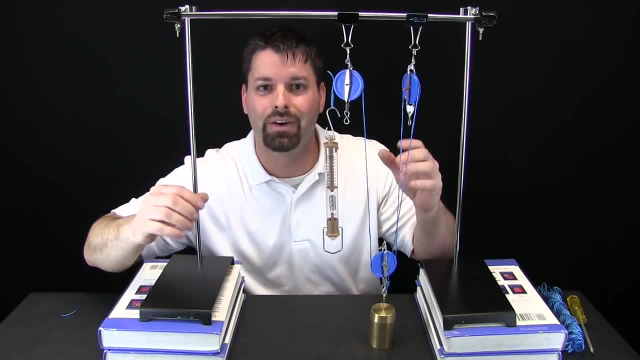 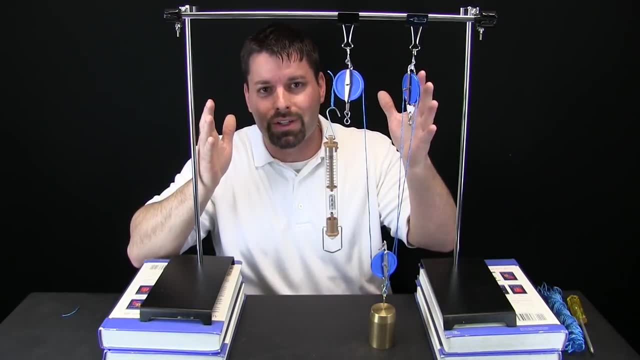 pulleys, or five pulleys together, Or six pulleys or seven pulleys all together, and had them working together, It would be very complicated to show you. Actually, scientists have designed a pulley system where all these pulleys are put together really closely. It is called a block and tackle. It is made to 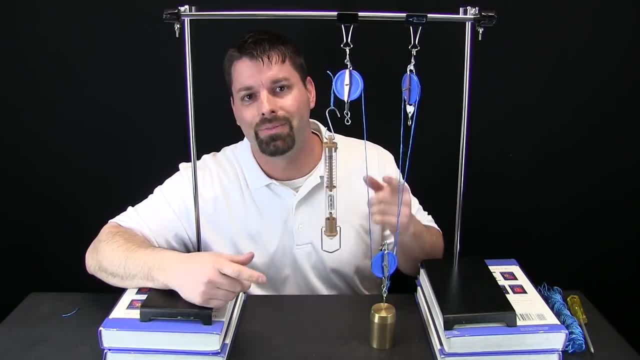 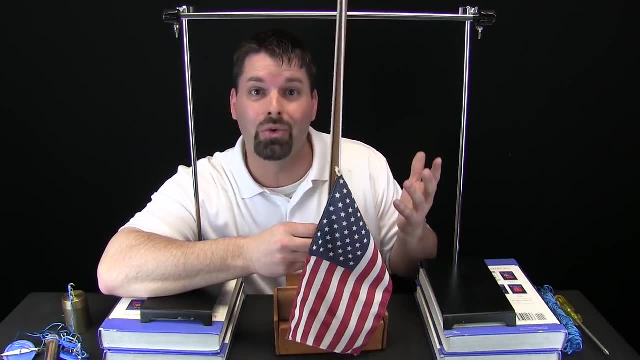 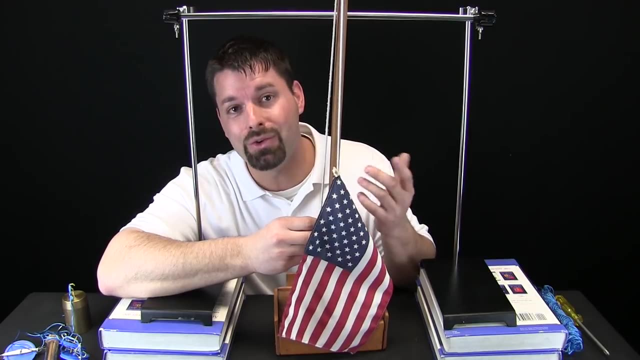 make lifting easier. It makes work easier. Simple machines like pulleys make work easier. Pulleys are simple machines. Pulleys really are all around us. Cars use pulleys, Boats use pulleys, Cranes use pulleys. Take a look around you and see if you can find pulleys.